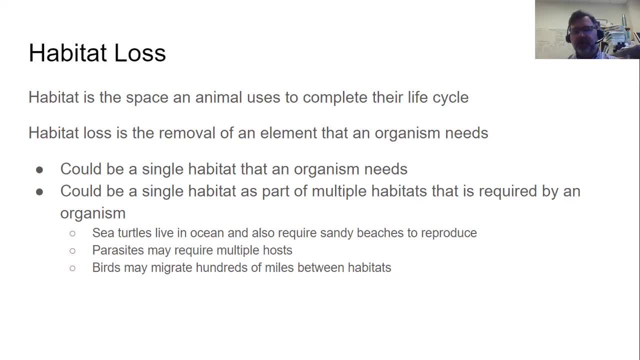 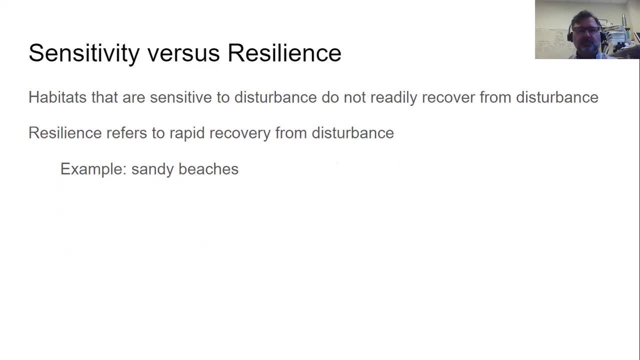 in Costa Rica and South America, And so habitat loss would be important for any of these elements in their environment. When we're speaking about habitat loss, we should think about sensitivity of a habitat versus its resilience, And this is a continuum. You don't have habitats that are necessarily. 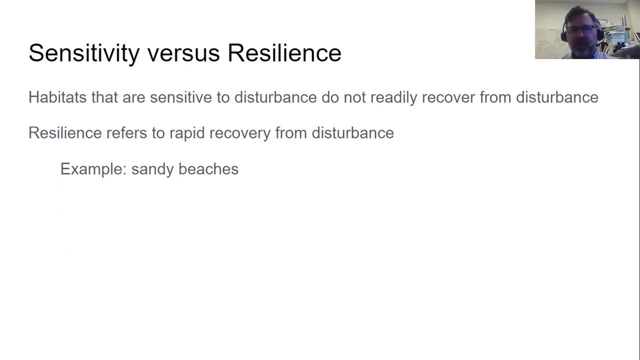 sensitive and those that are resilient. It's really a continuum. And when I say sense that habitats are sensitive, It means once they're disturbed, so bulldoze or turns into cornfield and then maybe abandoned. how quickly does that habitat go back to being what it was before? 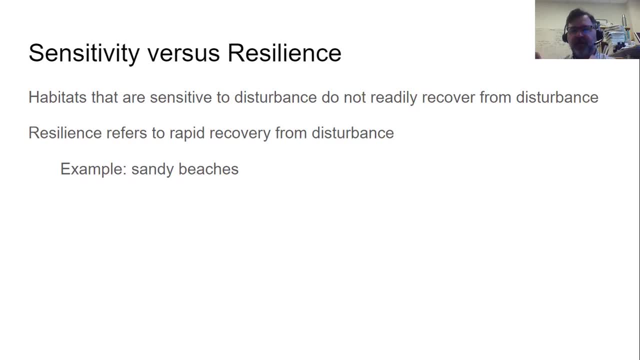 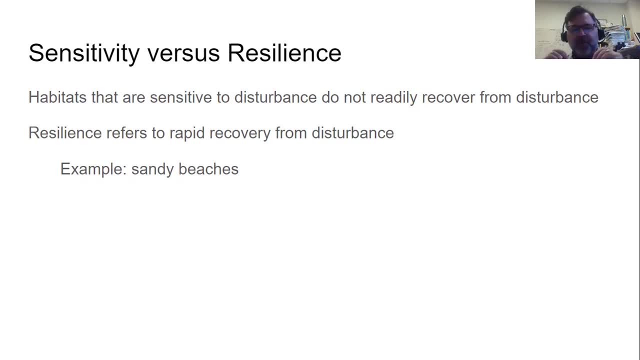 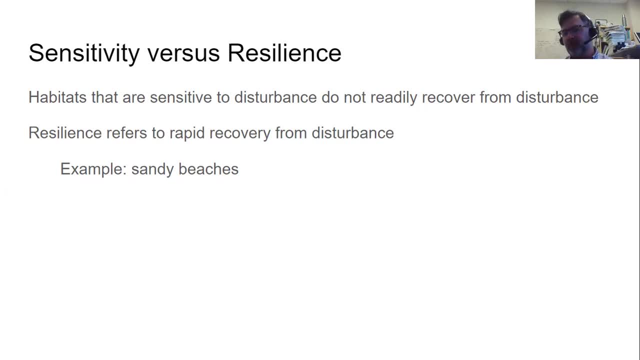 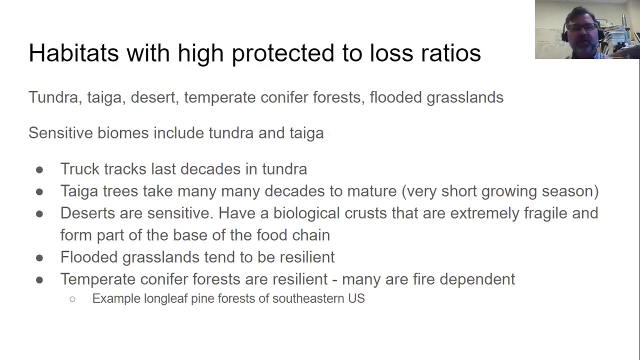 the, the people that drive the, the tractors that essentially comb the beach. it would go back to being a sandy beach. no problem, Okay, and we'll get to some habitats that are more sensitive than this. Okay, When we talk about habitats, because there are so many species, we're going to group. 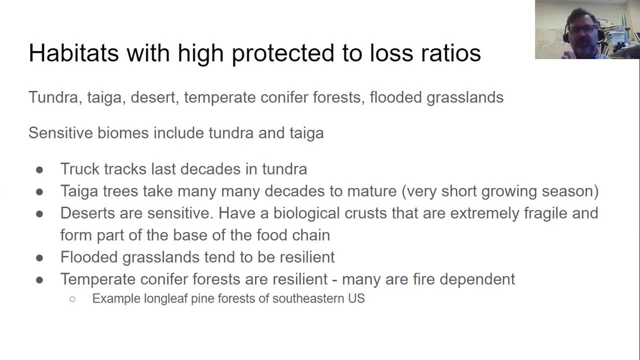 them together by biomes. So let's look at biomes with high protected to loss ratio. So these are biomes that have a lot of protection with very little loss. Okay, And this would include tundra, taiga, desert, temperate, temperate conifer forests. So this would 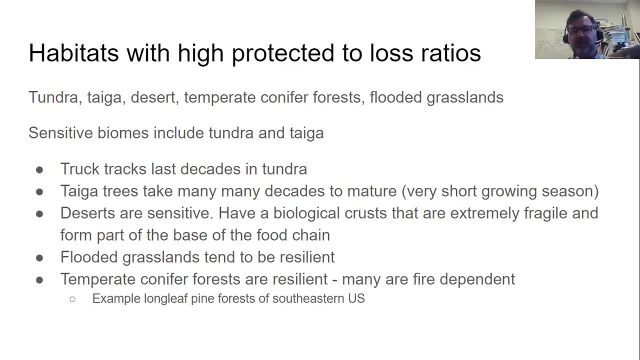 be conifer forests in the southeastern US and then out west, and then flooded grasslands. The sensitive biomes include tundra, taiga and desert. So, for example, truck tracks last decades in the tundra, which is pretty amazing. 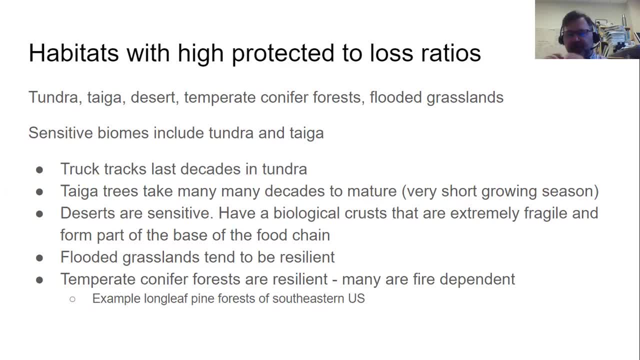 The taiga is now being rapidly deforested. I mean, a big chunk of it is protected, but it is being rapidly deforested. So this would be the spruce and pines up in Canada and Alaska. They're being cut down. 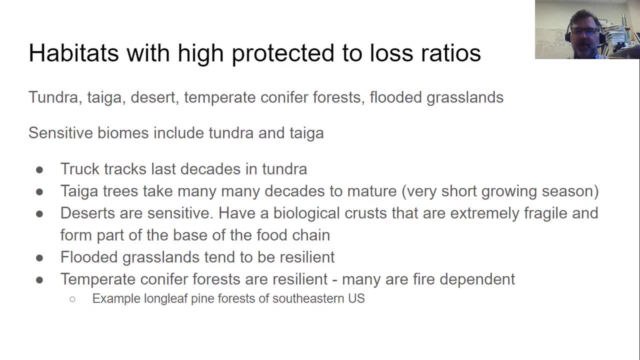 mostly for paper and timber products, And what you'll find is many of these trees take many, many decades. So in the southeast a longleaf pine may take 40 years to mature. It may take 100, 150 years for a spruce tree to mature to this point. So it's a very, very 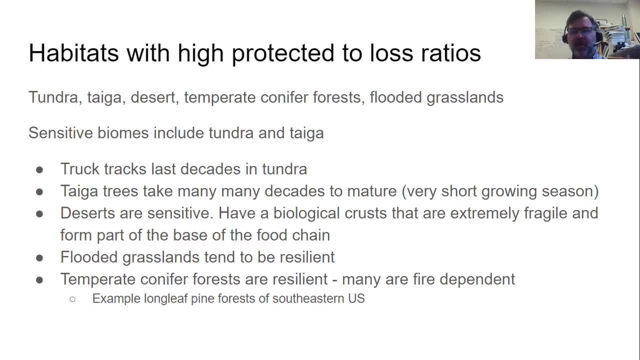 serious issue And we can't be sure, And there are a lot of studies that show that this doesn't necessarily mean the trees have to evolve or not evolve to the disappointed season. So there are things that are in the perspective of a year, a year and a half. 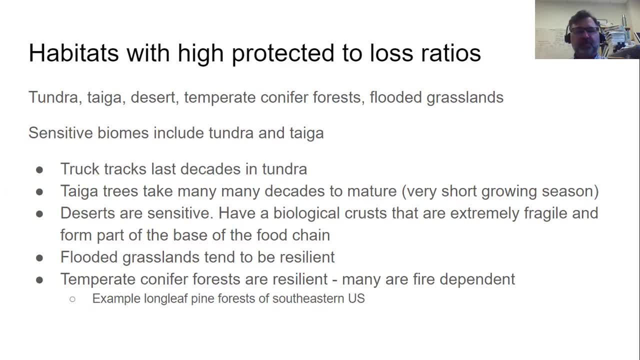 But what we can see is the growth of these trees, and what we're seeing is now 600,000 trees that are growing, And these are all trees that are growing with the same size, and that's because when you go more towards Alaska, you have a very short growing season. So the trees aren't able to grow very much in one single season. Deserts are very sensitive, And what makes them so sensitive is that they form these biological crusts, And these biological crusts are things like it's algae and that's a little. 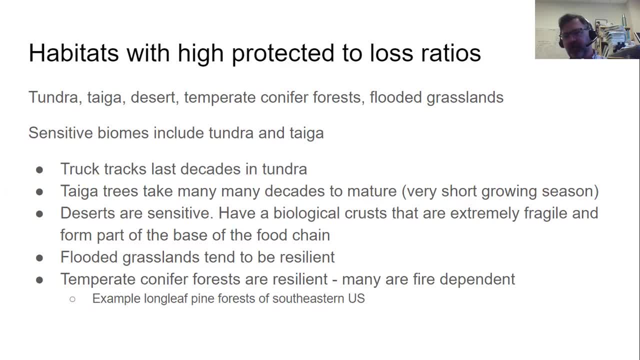 bit of a product we have in the culture, but we don't know how much a big tree can contribute, like it's algae and fungus, and sometimes it's lichens, and sometimes it's free-living fungus and free-living algae, and they tend to- and bacteria as well- photosynthetic bacteria. 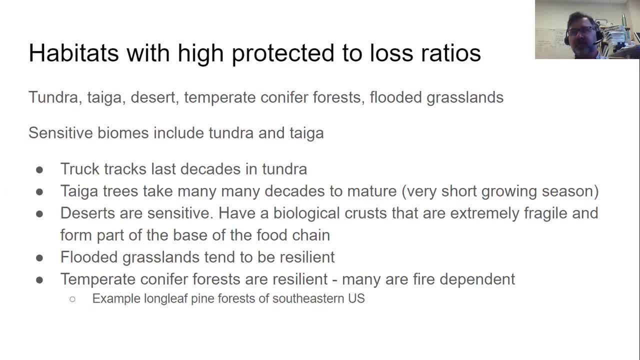 and they form this network. It's like a crust that can be easily disrupted by stepping on it, And these crusts are important because they form the base of the food chain. so they're, since they're photosynthetic, they're taking in carbon and that carbon can be used for little. 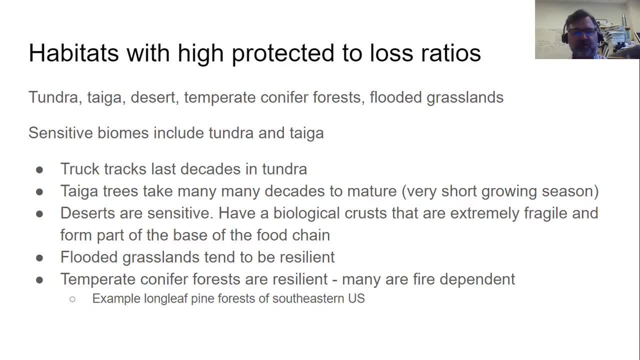 tiny things, and those little tiny things can be eaten by bigger things, and so on Flooded grasslands- we don't have those here in the US, but along riverbanks and riparian areas, um, these tend to be resilient, because if you're growing out on a riverbank, you tend to be. 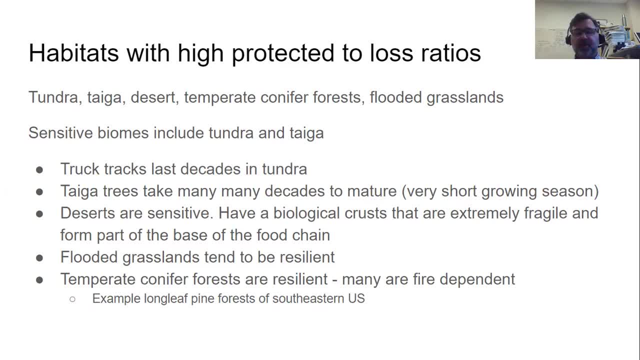 adapted to lots of disturbance. So along the banks of the Amazon, for example, and in South America and Venezuela, there are flooded grasslands all over and these tend to be relatively resilient. Temperate conifer forests are resilient, and again, we're just talking about like if a fire. 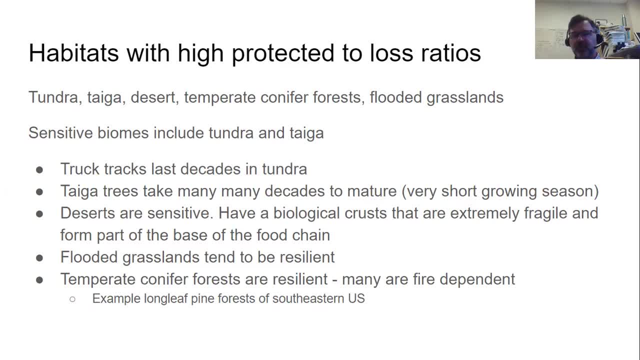 goes out, it's going to be resilient. So you know, if you're growing on a riverbank you tend to go through or you abandon agriculture. you can return those sites to uh pre-disturbance relatively quickly. And if you look at longleaf pines in the southeastern US, 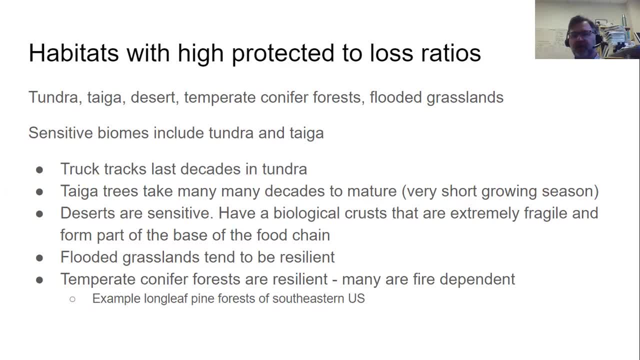 they're very resistant to fire. In fact, many of them, um, are fire dependent. So, uh, the leaves- I'm sorry, the seeds, um and the cones need fire to actually uh start their life cycle. And this is true out west as well, As bad as the? um fires are out west with the. 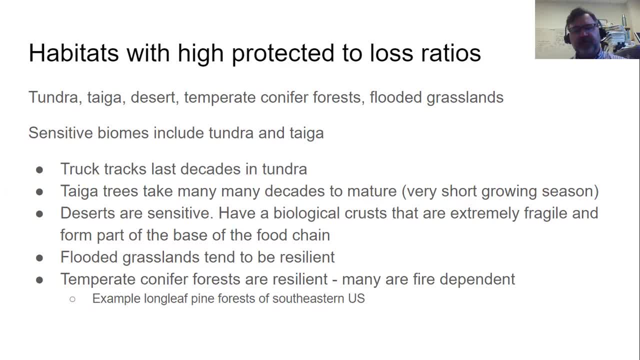 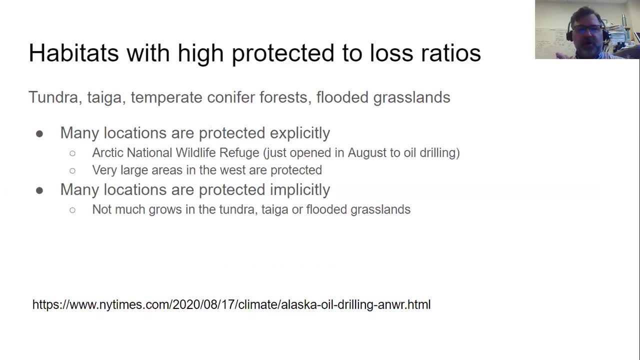 loss of life, the forest itself will bounce back. Okay, So uh getting into, uh drilling down to some of the uh biomes more explicitly? um, we have uh places that are protected, so why are these? the question is, why so much protection? Some of these are protected. 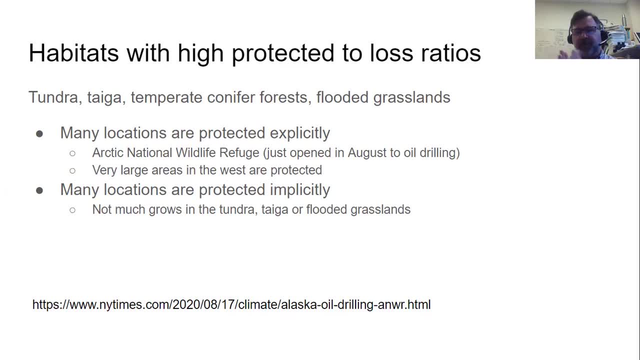 explicitly. In other words, they are protected because we tell them to be protected. And, for example, uh, the Arctic National Wildlife Refuge, huge refuge up in Alaska, uh, unfortunately they just opened it to oil drilling this past August. That'll be August 2020.. And large areas out west. 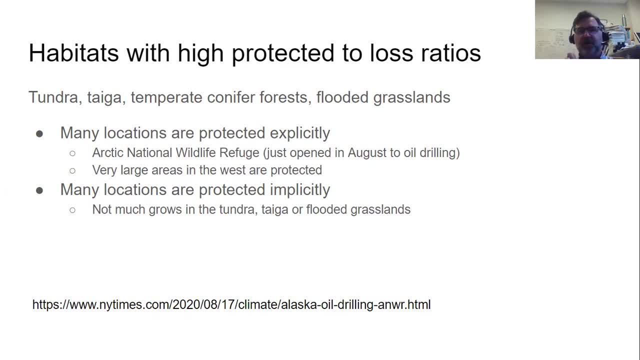 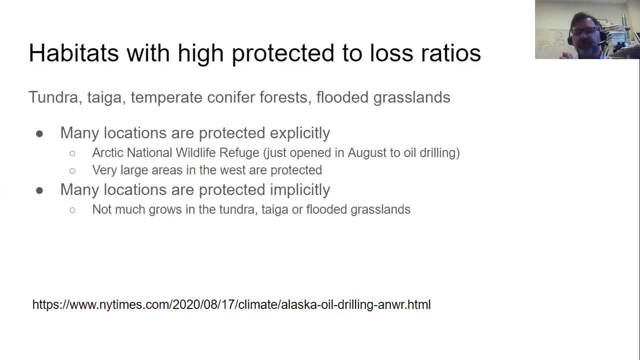 say bulldoze, and you can't uh build any permanent settlements on these things Uh and many locations uh are protected implicitly, And what that means is they may be privately held, they may be federally held, but they're not protected per se, And what I mean by 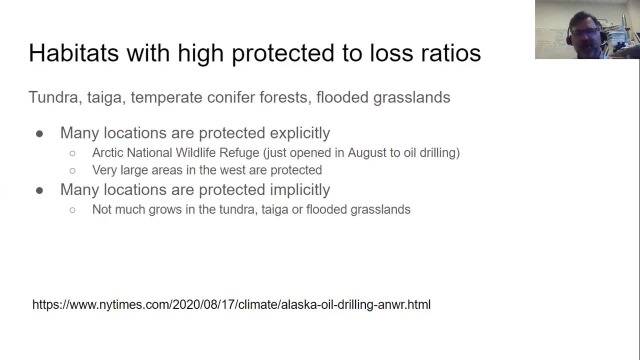 that is, it may just be a place where they're protected, but they're not protected per se, And what I mean by that is it may just be that, uh, you cannot, um, convert these areas to a land use that would be uh useful. For example, you're not going to plant corn or wheat or rice in the 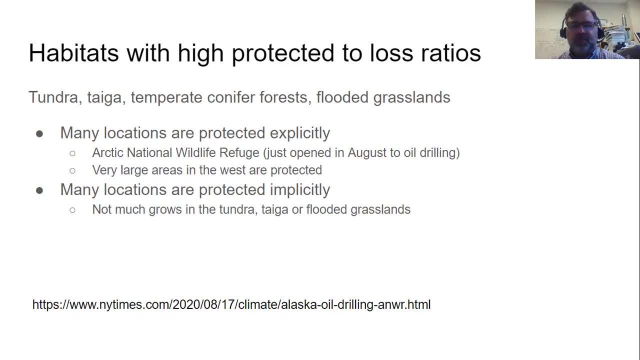 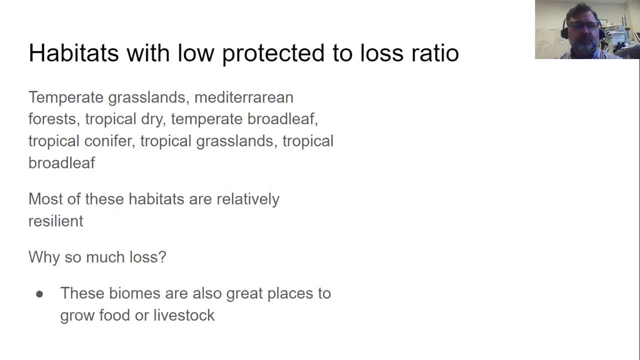 tundra. Um, so these, these places tend to be protected just because they're not useful to people. All right, Uh, habitats with low protected to loss ratio. So these are places that, um, don't have a lot of protection and have high loss, So many. 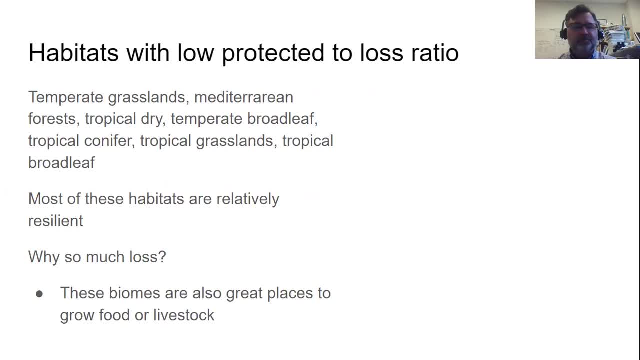 of these have been converted to something. some other biome as well- Non-natural biome, should point out. These include temperate grasslands, Mediterranean forests, tropical dry, temperate broadleaf, tropical conifer, tropical grassland and tropical broadleaf- what we just call rainforest. 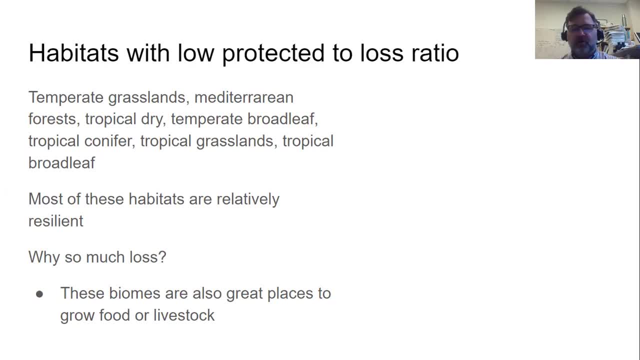 Okay, These habitats are relatively resistant- That's the good thing. So they've been converted over to something else, uh, such as farmland, pasture land. Many of these can be converted back to, uh, the original biome. Uh, why so much loss? So why this list? Uh, these biomes are also great. 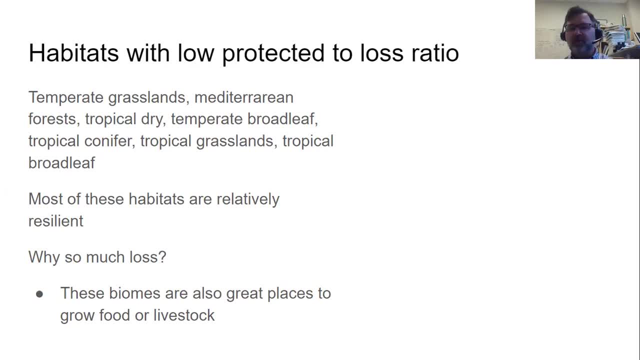 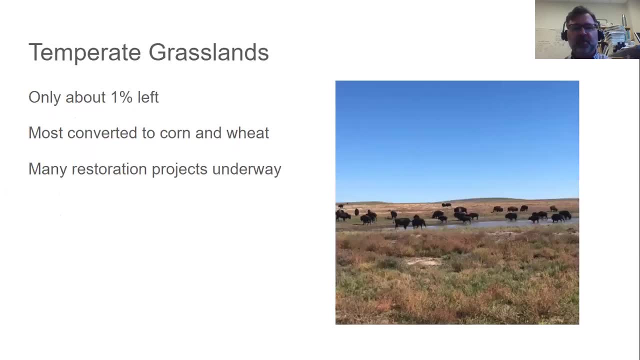 places to grow food or livestock. So I'll I'll go into some of these biomes in particular and talk about why, why so much is lost. Uh, the first one is temperate grasslands. There's only about 1% left of the original prairie in the 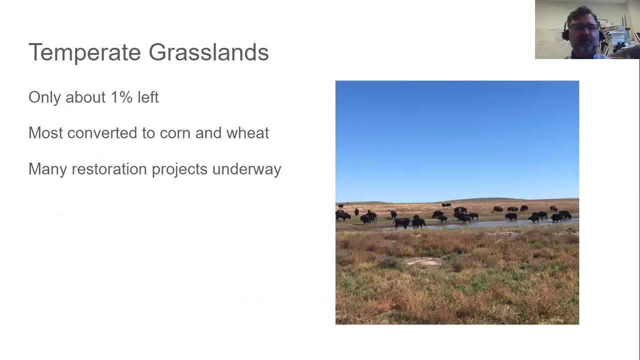 US. Where'd it go? Most of it's been converted to corn and wheat, as well as cattle ranching. The great news is is that there's lots of restoration projects underway And there's many endangered species in these habitats. There's several birds, several mammals, plants and 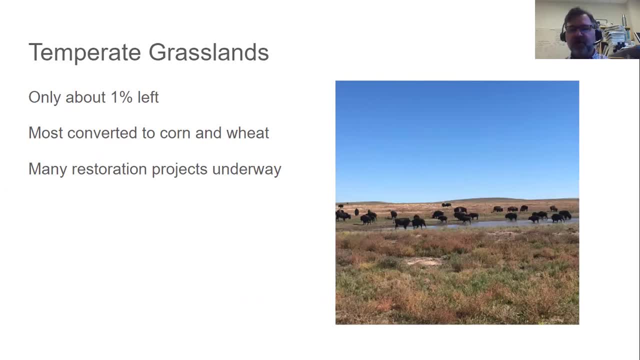 animals that are the on the endangered species list, And there's a lot of them that are on the species list from the prairie, And so this is a picture of bison And the bison population. just as the prairie is reduced to about 1%, so have the bison. 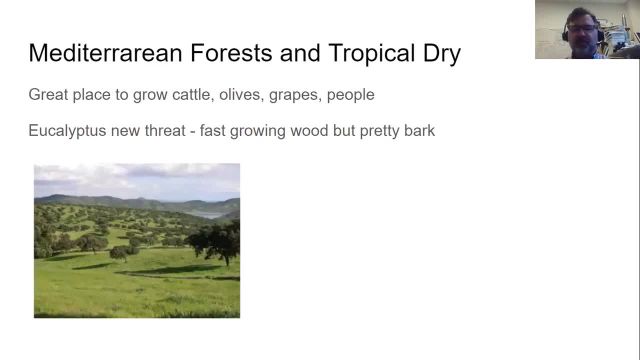 Mediterranean forest and tropical dry forest. So these are sites that have sparse trees and it's mostly grassland over top. These are great places to grow cattle, olives, grapes and people. So in the Mediterranean forest around the Mediterranean we've had human settlement there for tens of. 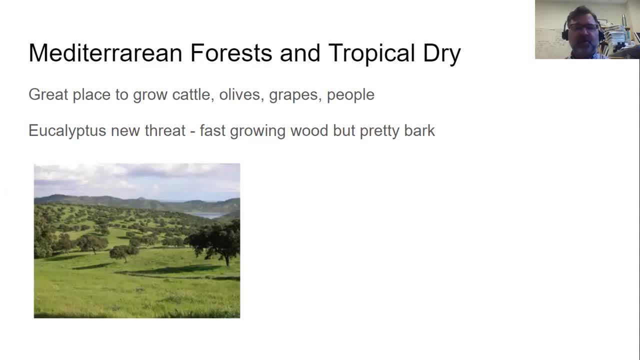 thousands of years. The only place where you find Mediterranean habitat in the US is in California And people really enjoy living there, right Napa Valley and great places to grow food. A new threat in the Mediterranean forests and the dry tropical forests is eucalyptus. This is a 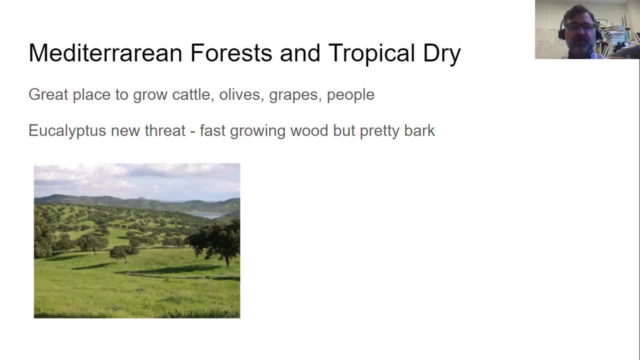 fast-growing tree that's used to make pallets and just serve any cheap wood that you need lots of. Eucalyptus is a great tree for that. Unfortunately, we're converting lots of dry tropical forests and Mediterranean forests into eucalyptus forests, which are not very diverse outside of their native. 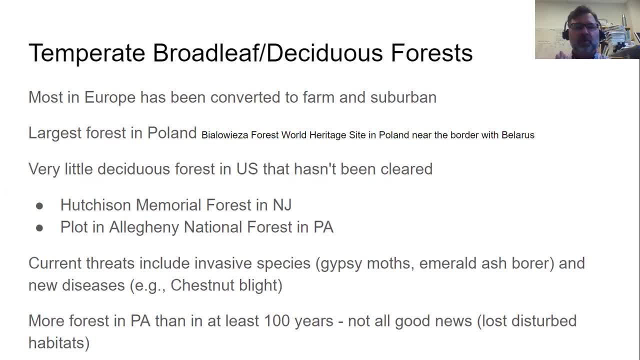 Australia, So spend a little time in temperate broadleaf and deciduous forest. This is where we are in Pennsylvania, And we're not the only deciduous forest. There was broadleaf forest in Europe. Most of that, most almost all of it has been converted to farm in a suburban landscape. There is 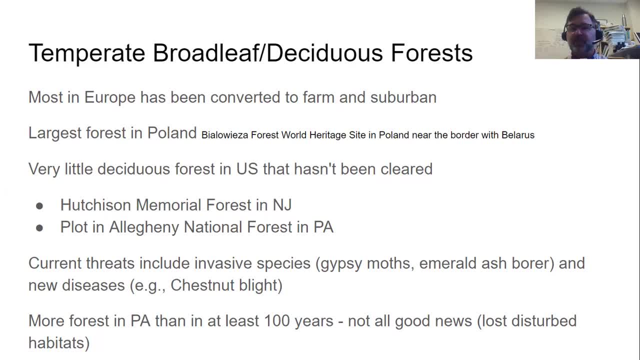 a huge forest left. It's the largest undisturbed forest- at least for centuries- in the world, And it's in Poland, near the border with Belarus, And I'm not going to attempt to say that name, and we just had a Wilk student there. 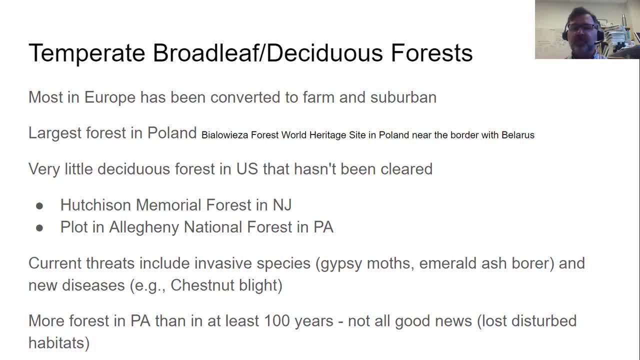 two years ago when she did a study abroad in Poland, and the forest there is just simply amazing. um, there's very little. it's not like we've taken great care of our deciduous forest in the US. there's very little of it that hasn't been cleared at some point. um, there are a few plots you can go. 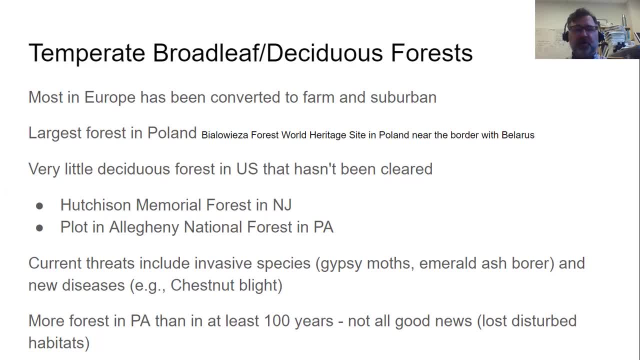 to that are hundreds of years old. you can go to Hutchison Memorial Forest in New Jersey. that's under ownership of Rutgers University. it's been studied intensively for decades and decades. and then there's a plot in Allegheny National Forest in central north central PA. that is. 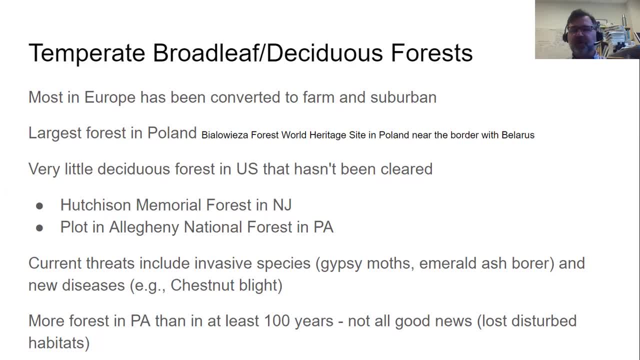 hundreds of years old as well. and then there's also some places where it's been difficult for people to get into and remove the trees, such as the Smoky Mountains. some of the steep slopes and the Smokies have trees that are hundreds and hundreds of years old. 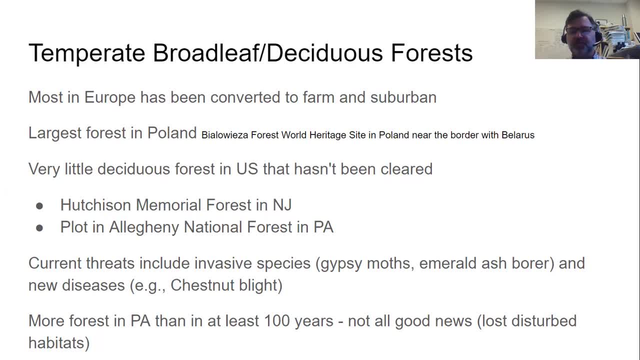 current threats to deciduous forests include the. in fact, the primary threats to deciduous forests include the. in fact, the primary threats to deciduous forests are invasive species. so you have things like gypsy moths, the emerald ash borer- uh, gypsy moths if. 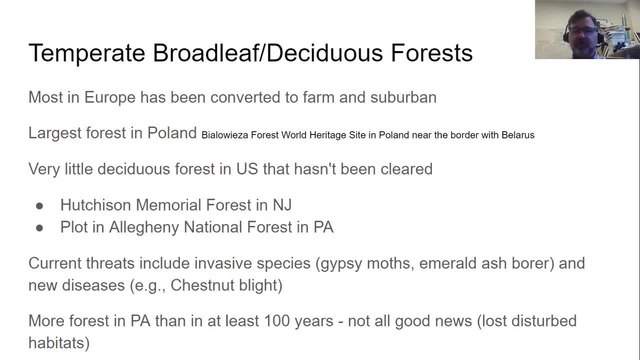 they defoliate an oak tree for two, three years in a row, it'll kill the oak tree. the emerald ash borer will kill ashes within a few months. in fact, Wilkes University had to remove 20 ash trees that were, looking at them, I'd say at least 40 years old, and they were all removed. 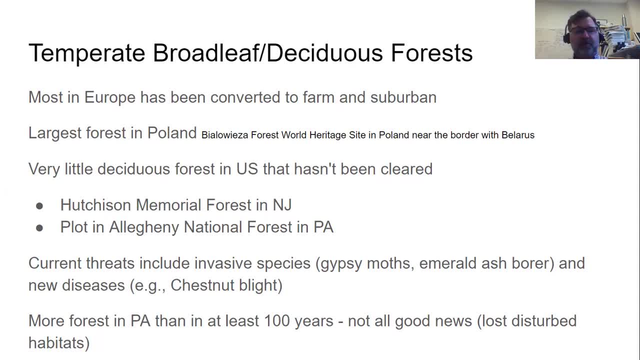 because the emerald ash borer and as well as new diseases. so the chestnut blight- most of the I would say the dominant tree in this area was probably chestnut- a lot of forests and the chestnut blight, which is a fungus, knocked it back and as far as I know there are no canopy. 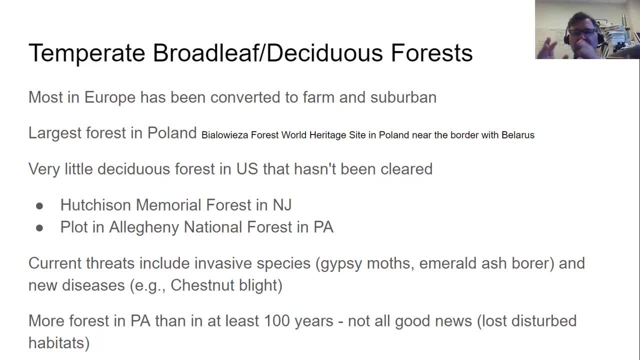 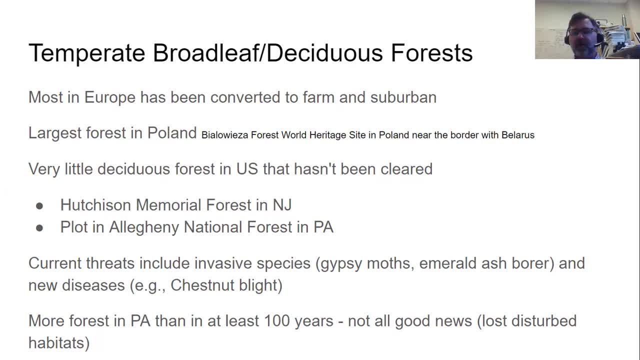 so you have these trees which might be hundreds of years old, but they have a very shrubby form and they get about half a foot in diameter, and then they get killed by the blight. so they're just not filling up the canopy like they used to. 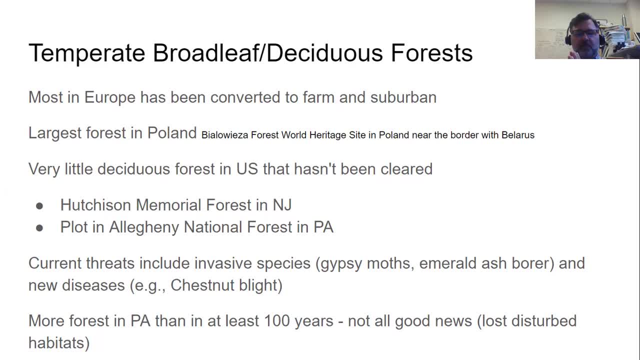 one interesting thing is that there's more forest now in Pennsylvania than there has been in at least 100 years, and- but it's not all good news- we've lost disturbed habitat. so what's happened in Pennsylvania was it was in fact, timber is our number one industry right now, but it historically 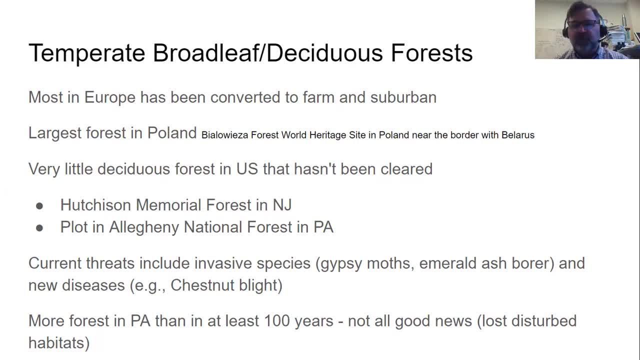 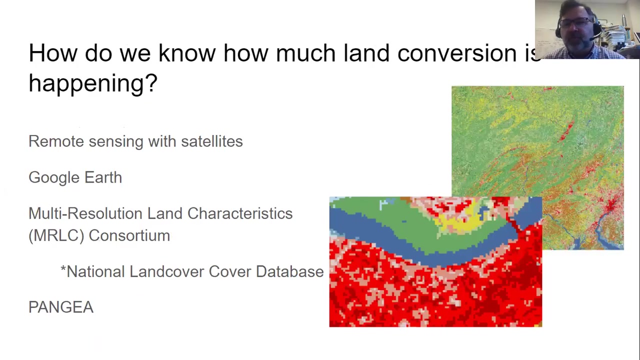 would have been farming, and many areas in Pennsylvania were converted to farm and pasture land, and much of that has moved out west, and so the forest have had some time to recover. what we are missing is disturbed habitats, and that's because of fire suppression. how do we know so, when we say there's one percent left of prairie, that 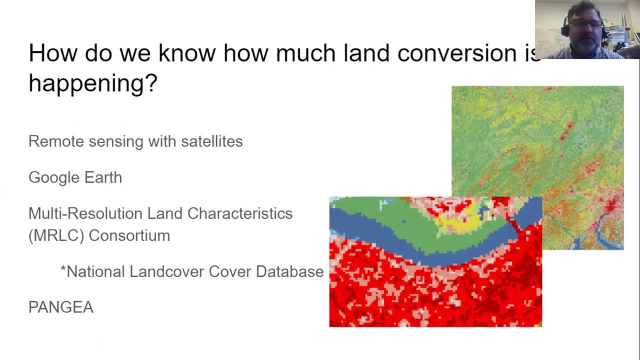 forest in Pennsylvania are increasing. how do we know these things? and the? the primary reason is: we use remote sandblasting sensing with satellites, And so Google Earth has proven to be a useful tool, And this is available to anyone. The multi-resolution land characteristics consortium. 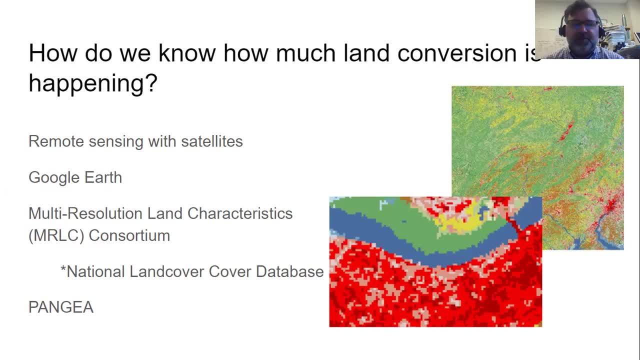 has a number of databases, And I think the most important one for monitoring land use is the National Land Cover Database, And so every couple years we take data from these satellites and they're available for public use. They're digitized and categorized into certain land uses. 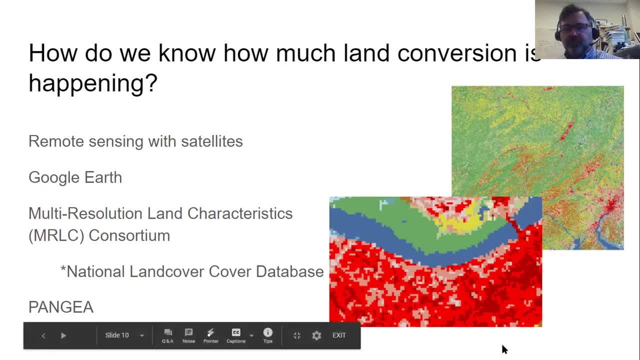 So this primary let's see here. So this larger, more fine-grained one is northeast Pennsylvania. Actually it's eastern Pennsylvania, This crescent shape here. So this is Scranton and Wilkes-Barre. You can see the Susquehanna. 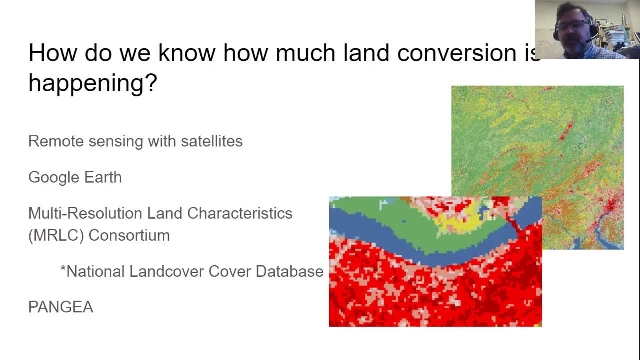 running into it. This is Philadelphia and Trenton And this is the Allentown area, So you can see the urban centers as well as what's heavily forested, such as this green area, And you can see the farmland in yellow here. Okay, So I say farmland, It's also.